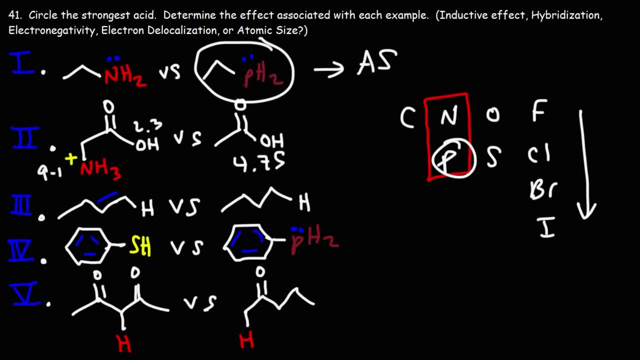 The NH3, that's like 9 to 10.. So this one is clearly way more acidic than acidic acid. Now what is the reason why the amino acid is more acidic than the carboxylic acid? So here we have a nitrogen atom That nitrogen is not. directly attached to the hydrogen, so atomic size doesn't apply here. The reason why this carboxylic acid is more acidic is because nitrogen is electronegative and it can pull electrons through the sigma bond by means of the inductive effect. So it's not just electronegativity but more. 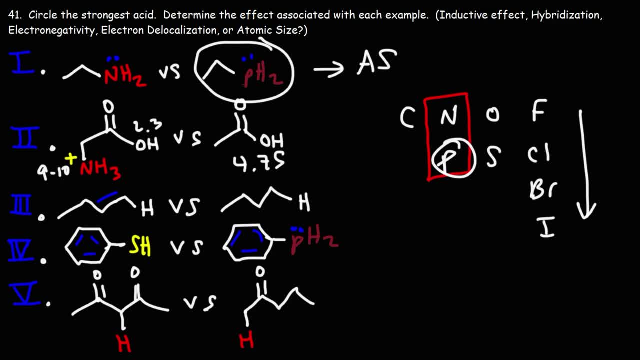 specifically the inductive effect, But electronegativity does play a role in that example. So the primary reason is the inductive effect. the secondary reason is electronegativity. So because nitrogen is electronegative, it can pull electrons by means of. 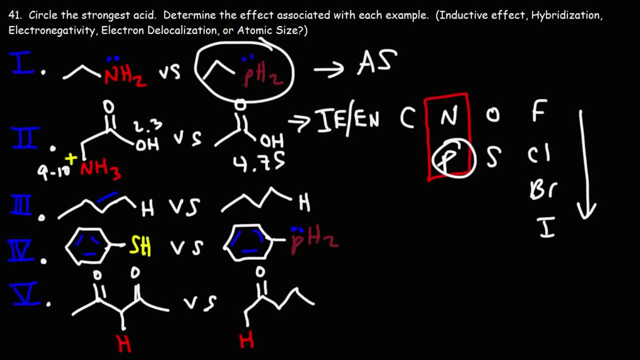 the inductive effect. But if I had a test, if this was a test- I would pick inductive effect over electronegativity. If the inductive effect wasn't there, then I would pick electronegativity. Number three: So here we're comparing two hydrogen atoms. 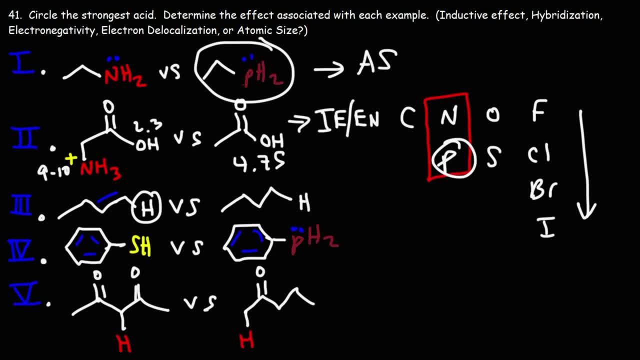 One is on a double bond, The other is on a single bond, So the hybridization is different. Here we have a hydrogen on an sp2 carbon, Here it's on an sp3 carbon. We know the alkene is more acidic than the alkane, So that's going to be the answer. The pKa for an alkane is 44.. For an 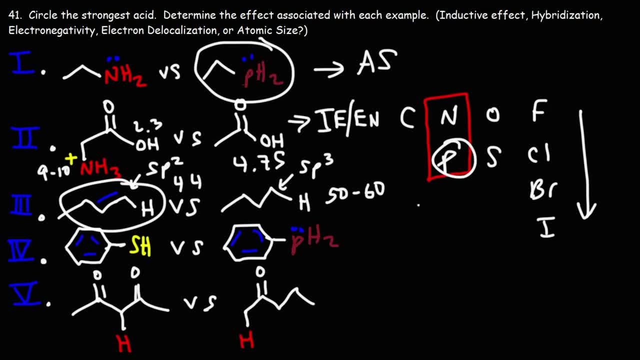 alkane, it's about 50 to 60. So the answer for this is: this is the strongest acid, or the stronger acid, rather, But the reason is due to hybridization Here this is the inductive effect and this is atomic size. Now for the fourth example. we're comparing sulfur. 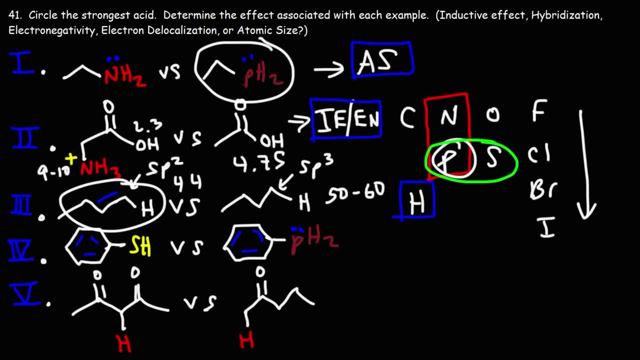 and carbon And phosphorus, When you're comparing two different elements in the same row. there's only one reason it could be, And that is electronegativity. Sulfur is more electronegative than phosphorus. Electronegativity increases to the right, So this is going to be the 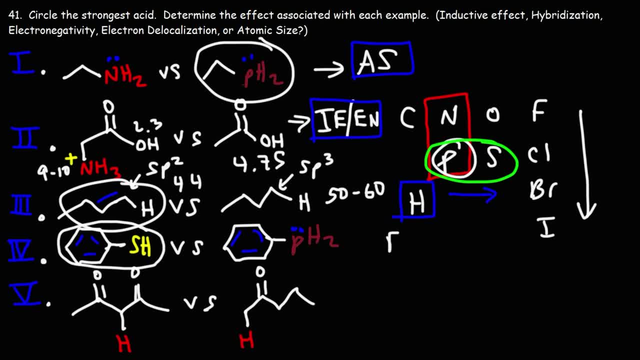 answer. So we're going to put En for the reason. Now for number five. We're looking at the alpha hydrogens. The alpha hydrogen next to a ketone has a pKa of 19.. This alpha hydrogen, between two ketones that are 1,3 apart, This is much less, It's 9.. 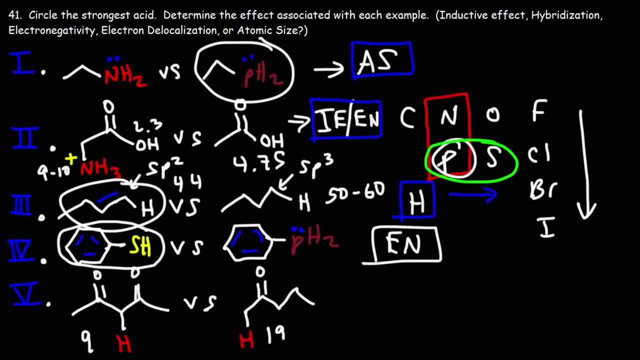 Now the question is: why is this so much more acidic? What is the answer? Is it the inductive effect? Is it hybridization? It's not hybridization because the hydrogens, they're both next to an sp2 carbon, So it's not going to be hybridization. 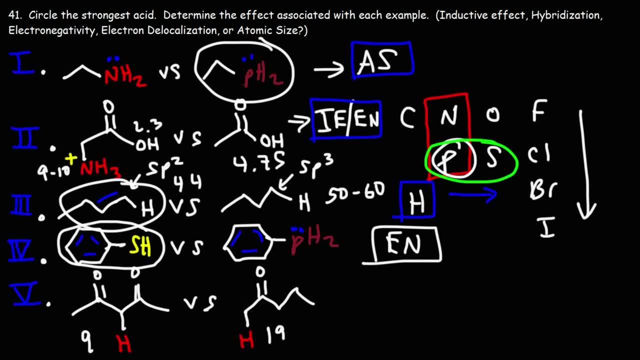 Is it electron delocalization? Is it atomic size? It's not atomic size, because we don't have any different elements: All the elements are the same. It's not electronegativity: The elements are the same. So is it the inductive effect or electron? 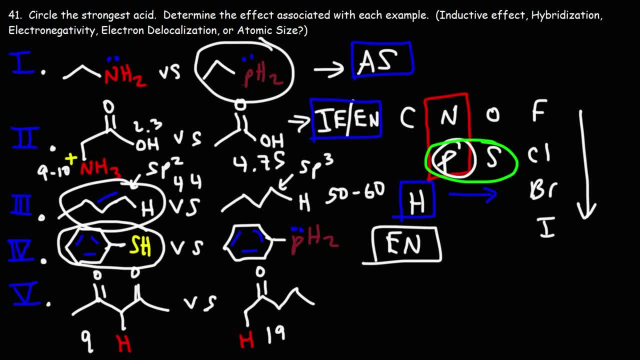 delocalization, The inductive effect. You're pulling electrons, the sigma bond, but electron delocalization, that's when you, that's when you start moving the pi electrons. if we were to take off the hydrogen, we would have a lone pair and this lone pair can move into the carbonyl group. so it's delocalized. 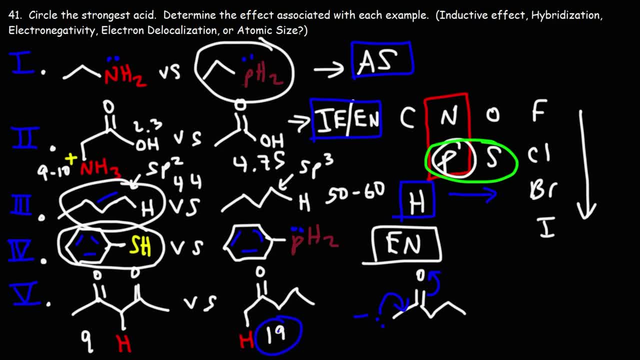 so the reason why this is relatively acidic compared to an alkane is because we can put the negative charge on an oxygen. that's why the pka is so much different here. but in this example we could put the negative charge on two oxygen atoms, even though the carbonyl groups 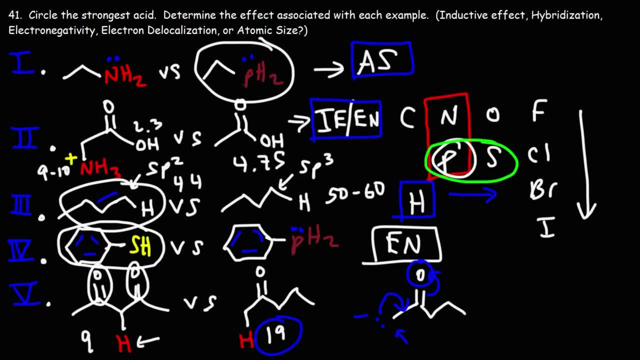 they do exert an inductive effect on hydrogen. that's not the major reason, that's not the strongest reason. the strongest effect has to do with electron delocalization. so the answer is primarily electron delocalization. the secondary answer is the inductive effect on hydrogen. that's why the pka is so much different here. but in this example, 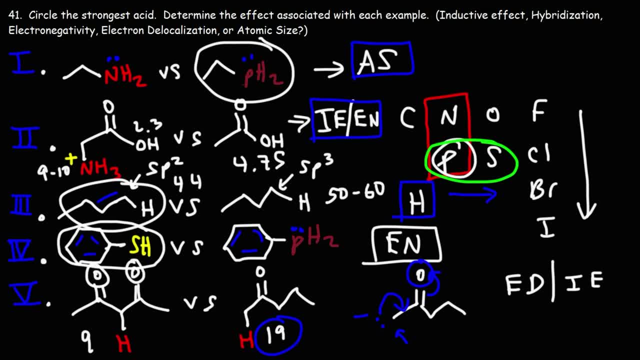 because these are electronegative electron withdrawing groups, so you do have some electronegative atoms here. you could put electronegativity as a third reason, but it's a minor reason because both of these have the same electronegative atoms, but this one has two of.